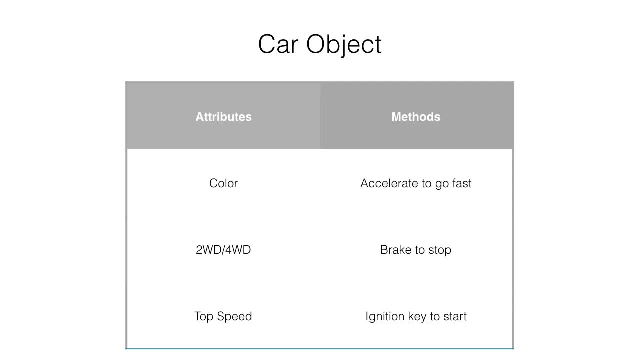 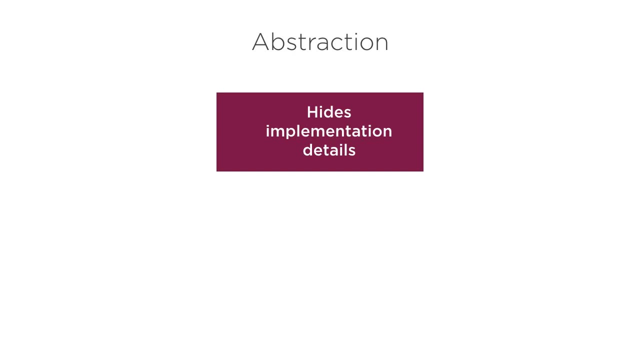 to press or operate in order to get a certain result. This is the principle of abstraction. Abstraction hides implementation details and provides you with a well-defined interface or controls to work with the object. In Java, abstraction is achieved by interfaces or abstract classes. Interface, as its name suggests, is an object. 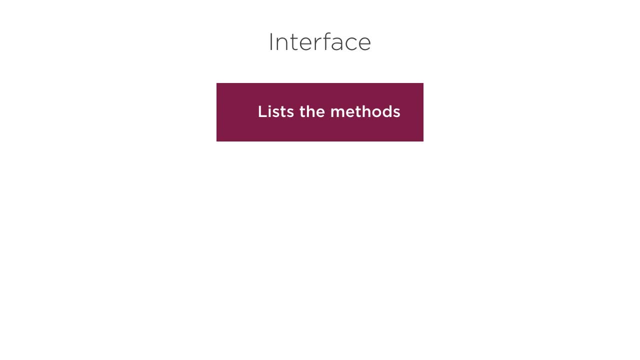 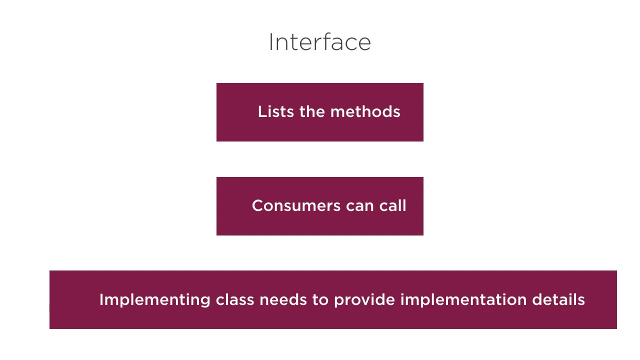 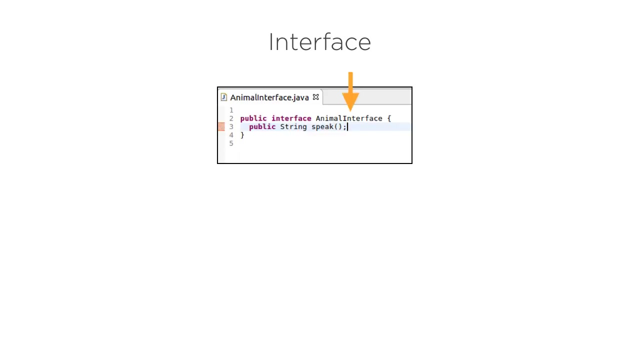 listing the methods available for consumers to call. A class implementing the interface needs to contractually provide the implementation of the methods in the interface. So, for example, here we have an animal interface which has a method speak. So any class implementing this interface will have to provide the speak method. So, for example, here is a dog class. 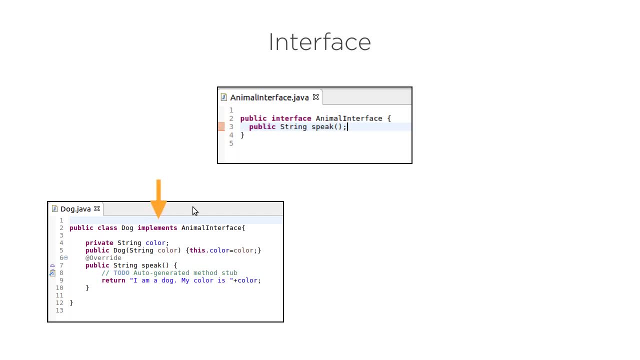 which implements. Implement is a keyword used to indicate which interface is this class implementing, In this case the animal interface. So this class has to create a concrete implementation of this method. Again, as we said that a class or object can have attributes. 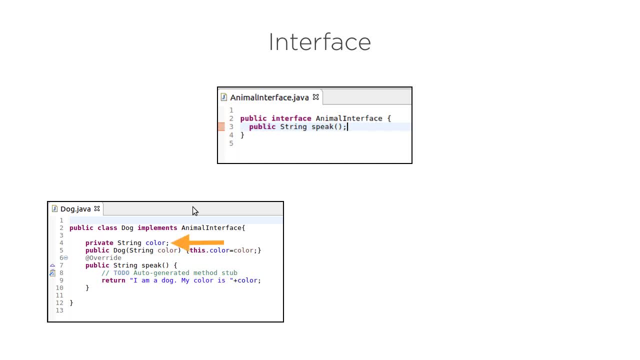 and methods. So here this dog class has an attribute of color and the method of speak. Here is another class, cat, which again implements the animal interface and implements the speak method, which it has to contractually implement because it is implementing the interface. Let's see it in action with a Java class. 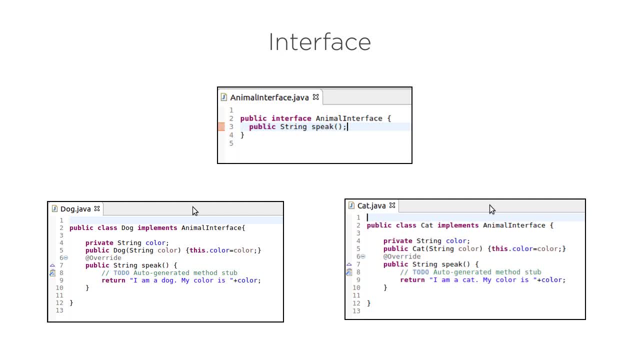 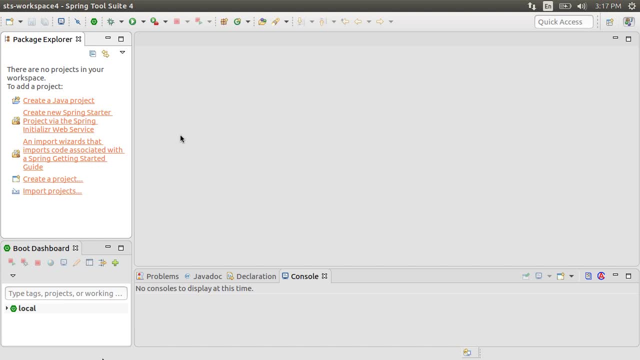 Now think of a Java class as a representation or a template of an object. Here I'm running Spring Tool Suite, a flavor of Eclipse, But you can download and use any IDE you want. IDE stands for integration, IDE stands for integrated development environment. You can use notepad also to write Java programs. 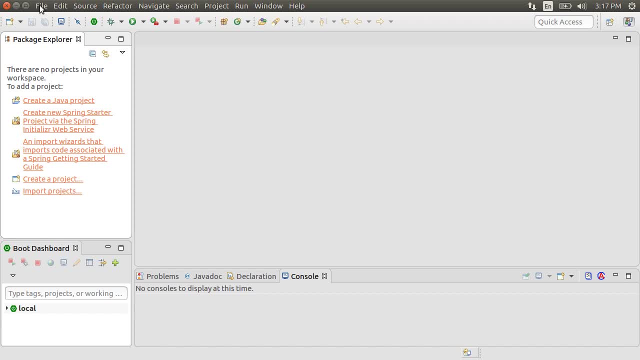 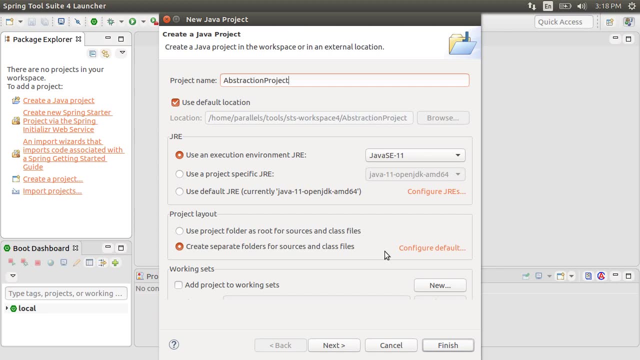 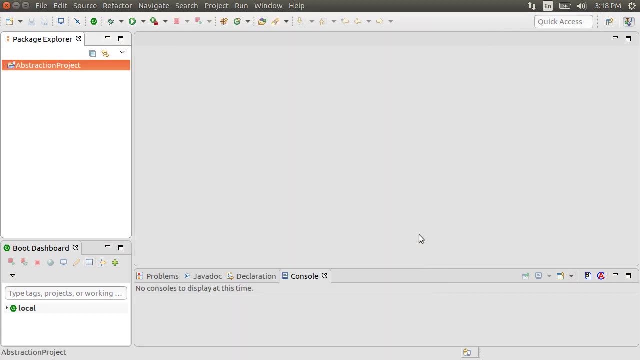 but an IDE makes it super simple. Let me create a new Java project by clicking new Java project. Let's give this project a name: abstraction project. Click next, Choose defaults and then finish. Now here is the project, Expanding it. we see the source folder. Let's right. 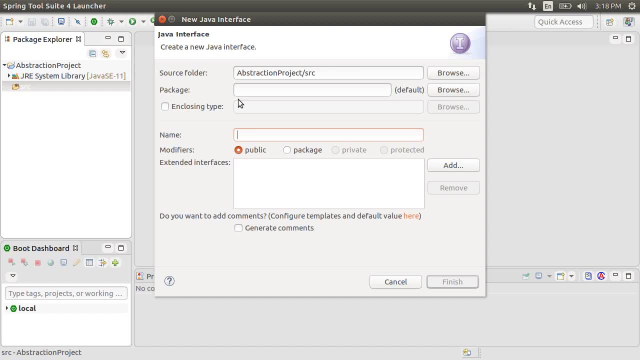 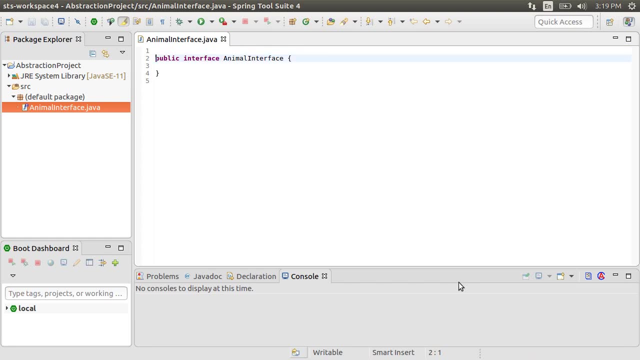 click and choose new interface. Give it a name: animal interface. Click finish Inside. let's create a single method: public string speak. An interface needs to have its methods as public. It just has the method definition, as the implementation will be done by the implementing class. Let's now right. 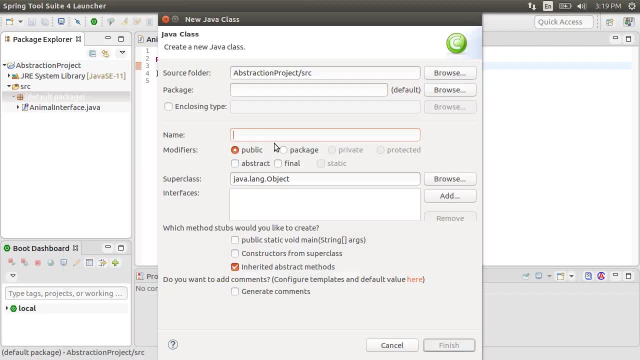 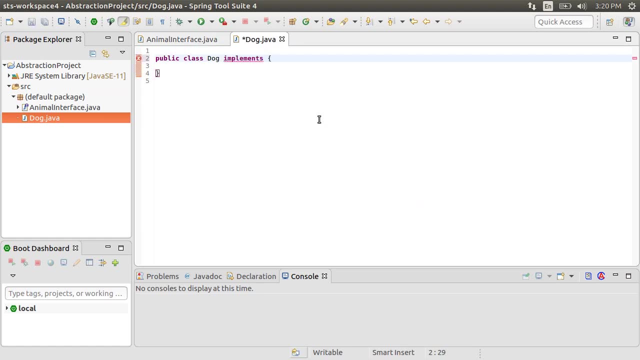 click and choose new class. call it dog. Now lets have this dog class implement the animal interface. by using implements animal interface. The IDE draws a red wiggly. That is because we are implementing the interface, but we have not provided the implementation of the speak method. 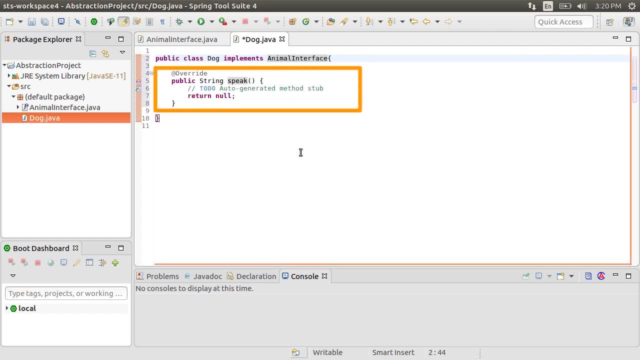 Let's click add unimplemented methods and here it generates it for us. The add override annotation indicates to the compiler that the annotated method must override an ehxisting supertype method, Either from an interface or an abstract base class. Now a class or. 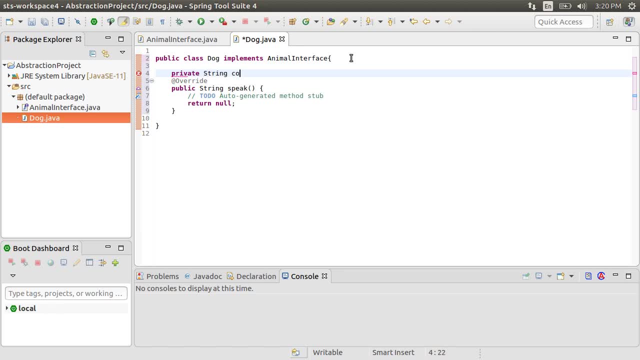 object can also have attributes. Let's add a private attribute: color. Adding the private keyword prevents this variable to be visible to outside classes and can be only seen by this dog class. So for the method implementation, let's just return. I am a dog, my color is. 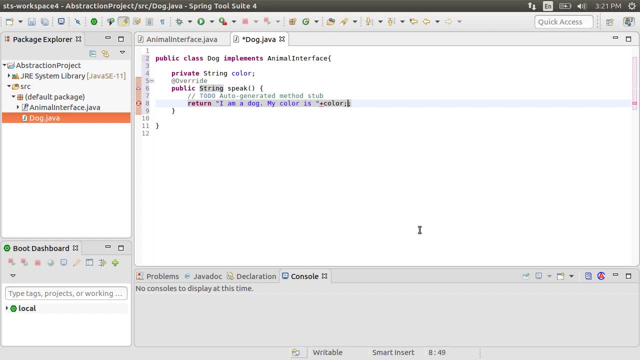 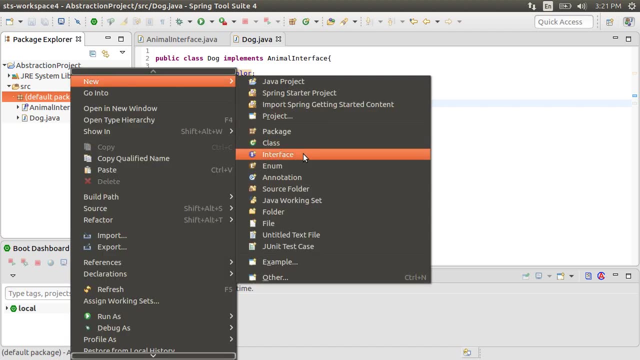 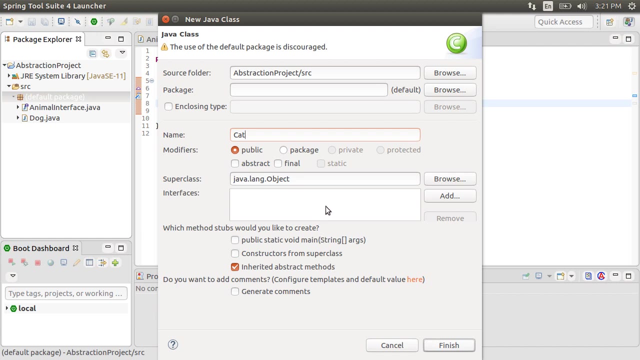 and, using a plus sign, concatenate or attach the color variable. Let's create another class by right clicking and choosing new class. call it cat Now. previously we added the implements animal interface manually. We can have the IDE do it for us. Click on add- choose animal. 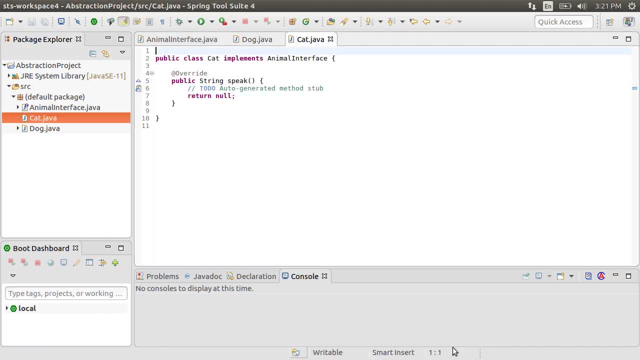 interface and click finish, And here it generates the implements keyword as well as the method steps. Cool, Again, let's create a private string variable color. Now let's create a constructor public cat pass in the string color and inside say this: which refers to the instance color variable. 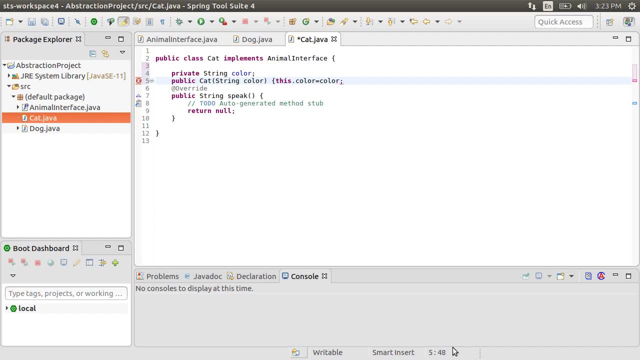 and assign it the past color. So when we construct a new object from a class, Java calls a constructor by default a no args constructor. But if we have to initialize a variable we can create our custom constructor passing in the variable to initialize.